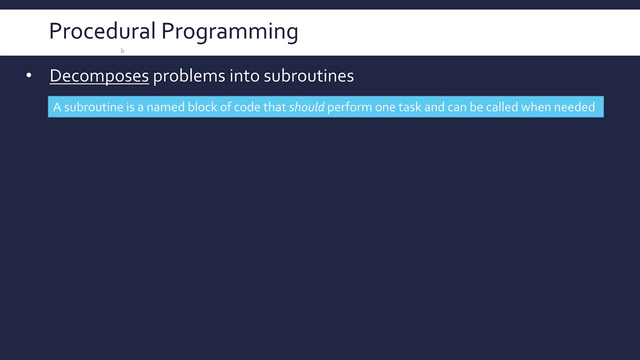 oriented programming that includes functions and procedures, or just subroutines, to give it a more general name. Now, when we're designing procedural programs, we sometimes make hierarchy charts- or most likely in an exam you will have to deal with hierarchy charts. So these are very simple diagrams representing how subroutines relate to. 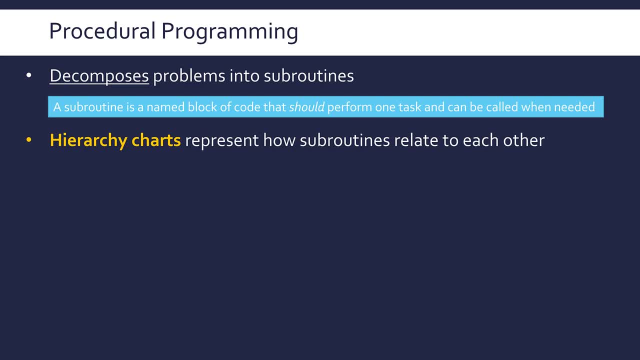 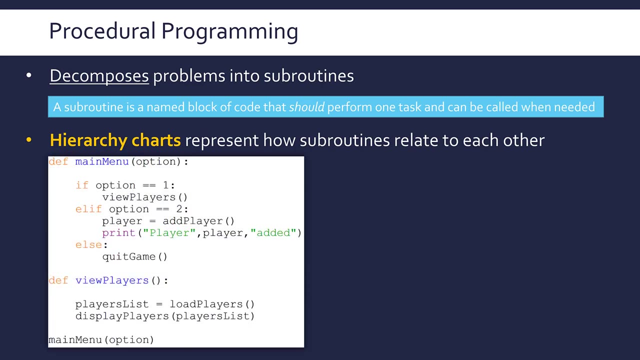 each other. So mostly the order in which they call each other, because a complicated program with lots of subroutines will be, they'll call each other, they'll become nested subroutines and so hierarchy chart is meant to show that connection. So just to give you an example, here is some Python code I've 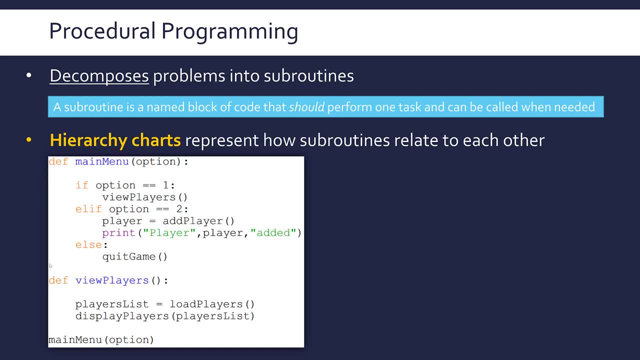 got two subroutine definitions: main menu and view players. I've also got a fair few subroutine calls, so I've not shown the definitions of most of these because it's just a bit of example code. It's more like a video game where I've got a main menu. I'm calling different options in this main menu is my thinking. 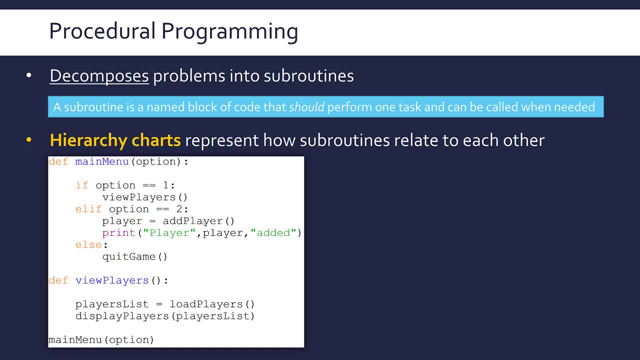 Well, how would I put this as a hierarchy chart? So, what you do, the first box you draw and it will be a rectangle with the identifier of your subroutine. so the name of your subroutine, The first one you put down at the very top, is the. 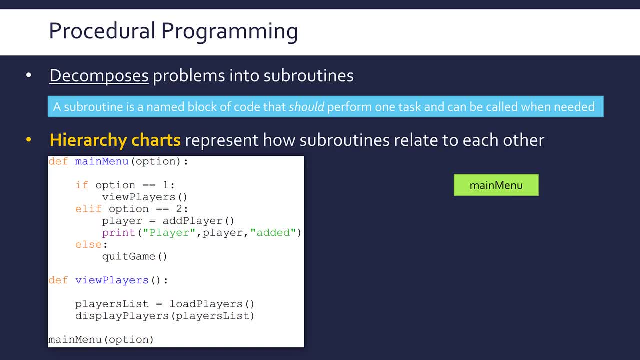 first subroutine to get called in this code. So in this particular bit of code the first line which gets run is a main menu at the bottom, which is a subroutine call and it's a call of main menu. So I'm putting down main menu as my first option. It's not because it's my first. 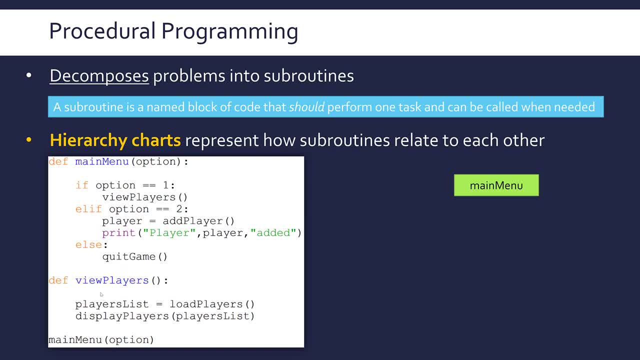 definition. it's just coincidence that it is. The definitions aren't looked at until we actually call one of them Okay. so it's not the top definition, it's a first one being executed Now, as a word hierarchy would suggest, we are sort of working our way down and looking at what comes next. 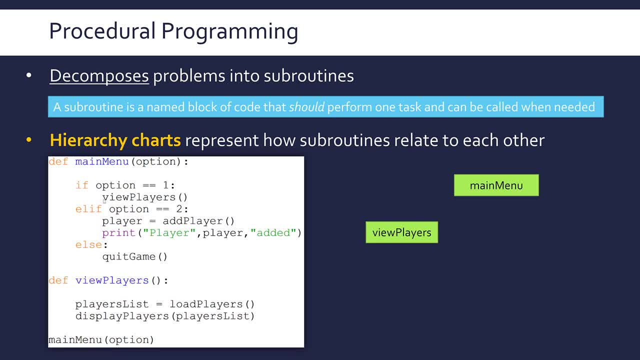 So inside main menu, once it's been called, what other subroutine calls do we have? Well, we're calling view players, which I have got defined here. We're also calling add player, which I haven't shown here but is another subroutine we can tell because it's it's got the call structure. we're familiar with the name. 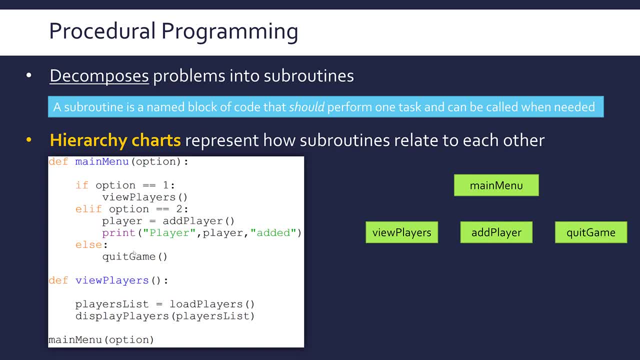 then brackets and we've also got quick game. Now print is a subroutine. we don't really care about it because it's not a user-defined one. it's built in and so we don't put it down, usually in a hierarchy chart. Now we connect these up. 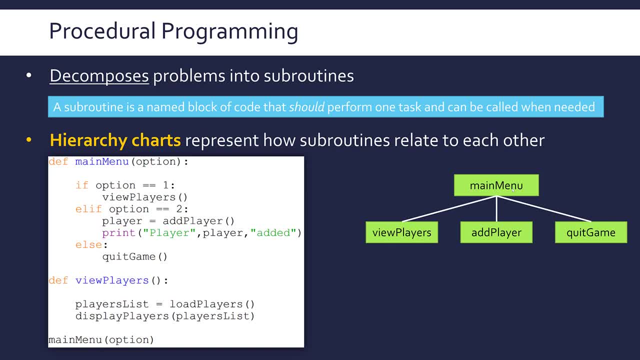 just with lines. so the lines, not an arrow, just a line. it's connected up to the subroutine which called it. So we can start to see this hierarchy. we start main menu. main menu can then call one of these three subroutines. Now it is one of. 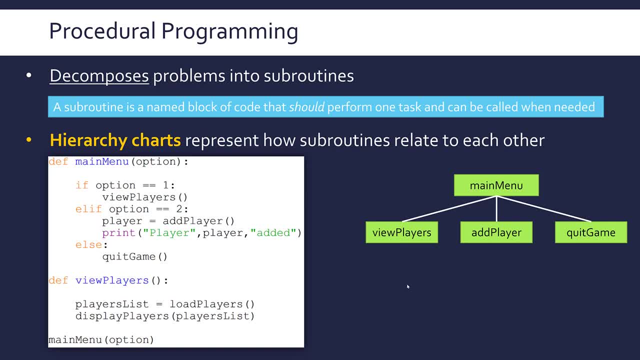 those three right. one gets called at a time. it's not a chain, because it's an if elif else structure. only one is getting called at any given point, And now the structure just builds and builds as you have more complexity. So I've only shown. 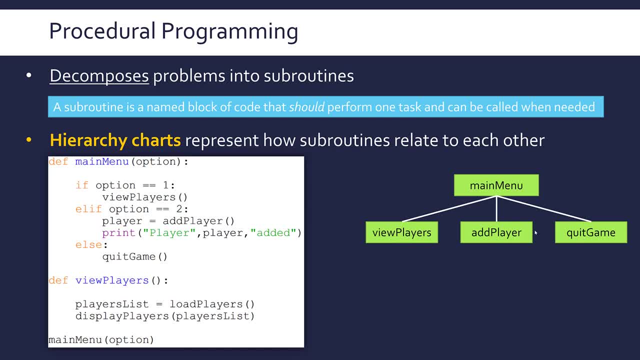 another definition for view players. I haven't shown add player and quit game, so let's assume they haven't got any other subroutine calls And view players have also called a subroutine called load players and another one called display players, and so again they sit under view players. they only get called within it. 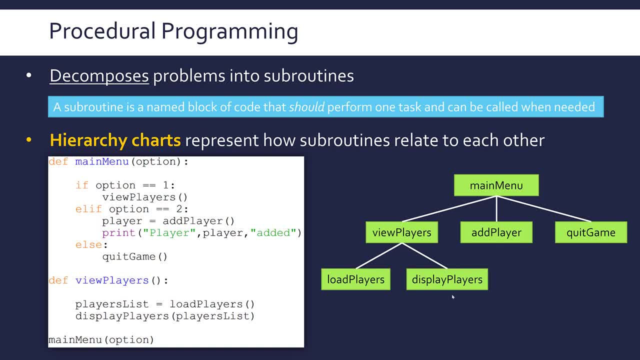 and so there are below it in the hierarchy chart. Now, this is quite a typical tree structure. it's not always a pretty tree like this. it will you start at the top with your first call, but sometimes you might get lines going back on each other. you might have lines connecting up. you might have it kind of 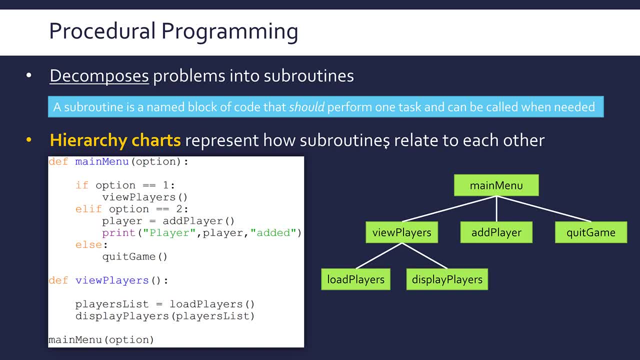 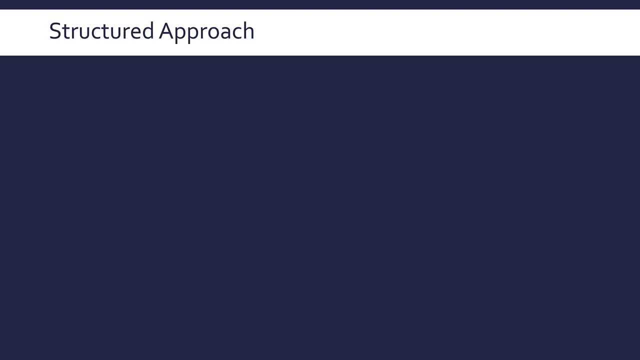 deviating a little bit. it just depends on our structure. it's not always as picturesque as this one Now. procedural programming is a paradigm, but so is structured programming, and it's a bit murky which one came first. it's not that important. we're going back to the 1950s- 1960s at this point, but you should be. 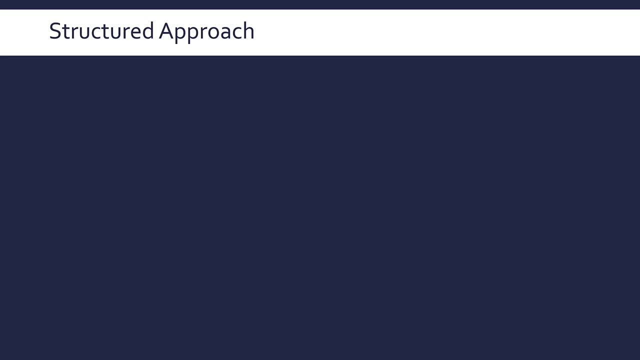 when you're coding in a procedural way, Make your code as structured as possible, and the structured approach as time has gone on has included a few key characteristics which are a sign your program is well written. essentially, so should be aiming to include these in any code we're writing. So key aspects of this include just having a very clear 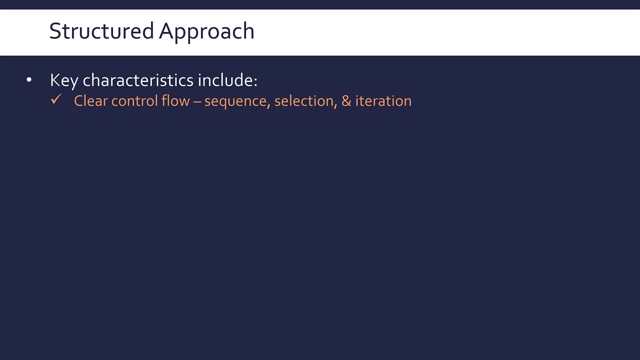 control flow. Our three basic constructs in procedural languages are sequence, selection and iteration. you should be using those as much as possible Now. in the early days of programming, go to statements were really popular. this is where you would jump around between different lines. you could just go go to line whatever and it would just go back. 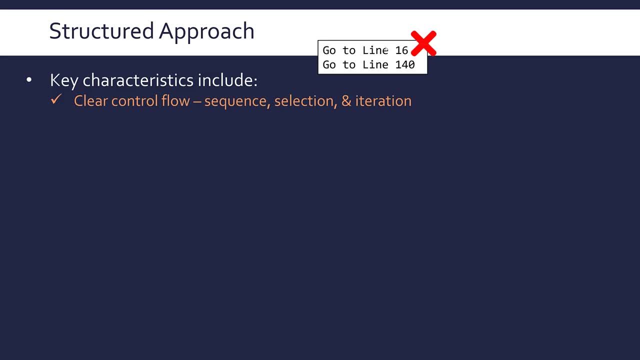 to that line and keep running and over time this would get really, really messy and really confusing. The instruction of selection and iteration in particular was meant to make this a lot clearer, so you're not just randomly jumping around all the time. it's a clear block. Recursion is kind of a fourth programming. 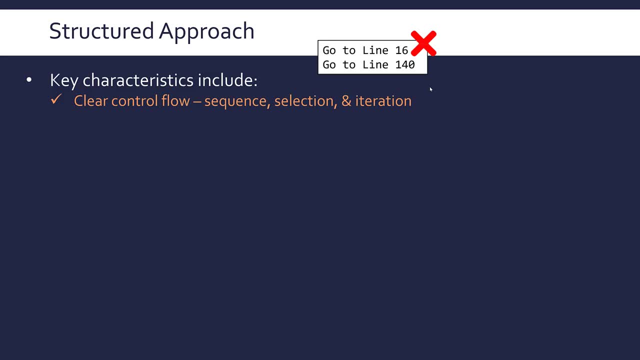 construct which, if you're a purist for structured programming, you would try and avoid. Part of the reason why structured paradigm and procedural oriented programming are really the same thing nowadays is because of subroutines, So we should be using subroutines with clear interfaces. 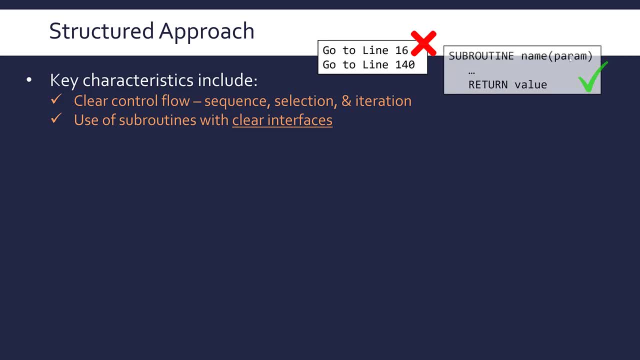 Now this isn't always ironically clear. The interface of a subroutine is what you interact with when you call it. So when you call a subroutine like name, in this case, which is the name of my subroutine, you're going to give it a parameter. so the parameter, or parameters, is your input to that subroutine. 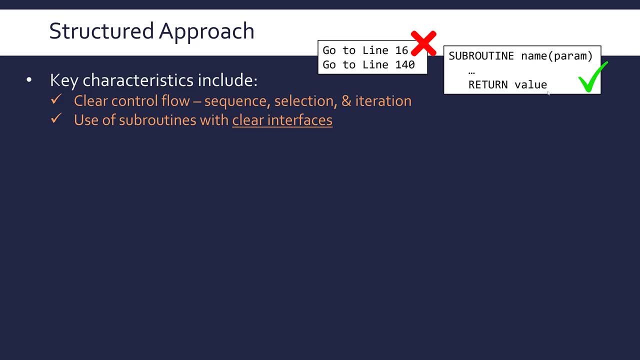 And it's part of its interface, and also, if it returns a value, if it's a function, you could consider that part of the interface as well. So the point is, you've got this clear definition of what parameters you need and what's going to get returned. That's what you need to focus on. you don't need to worry about what's. 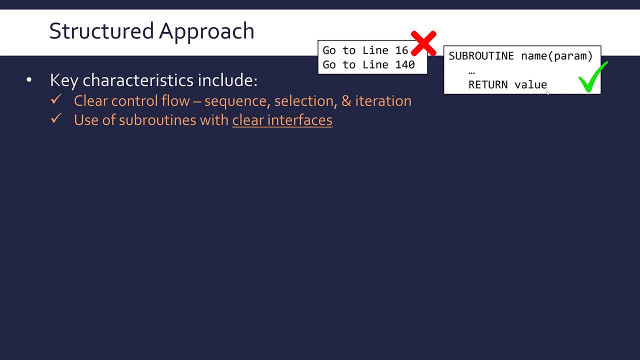 inside the subroutine, as long as you're happy with the interface. And in relation to this, subroutines should be loosely coupled. This means one subroutine should not negatively affect another subroutine. They should be very independent and almost disconnected, The only connection being through the interface. In practice, this means minimal use of global variables. If 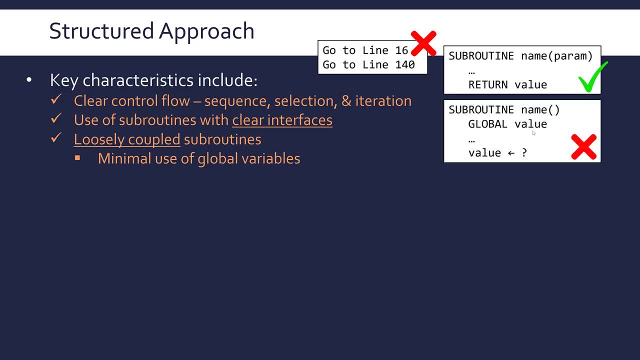 you've got a variable which is global. this means it applies to every other subroutine in that program. And so as soon as you use a global variable, when you change it, that's when it can start to affect another subroutine, because another subroutine might rely on that value which is now being changed. 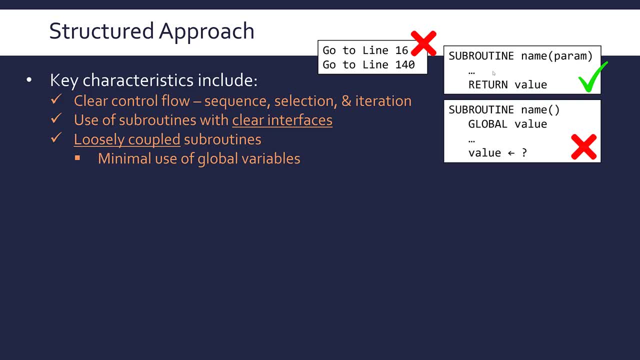 Whereas if you've got parameters and local variables and return values, it reduces the risk of it affecting another subroutine because it's contained just to that subroutine call. When you've got loads of subroutines, you're meant to use modules to group them, And now a module can be a separate code file. it could be a. 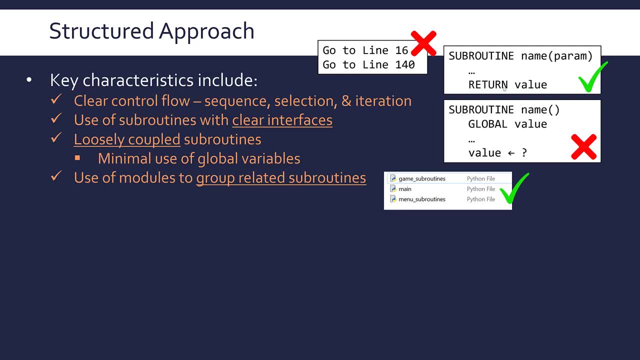 library. it could be a section within your code, but a way of grouping related subroutines makes things more logical, makes things more structured, And just consistency as a final point is really important. So consistent identifier names, consistent style of programming, consistent use of common. 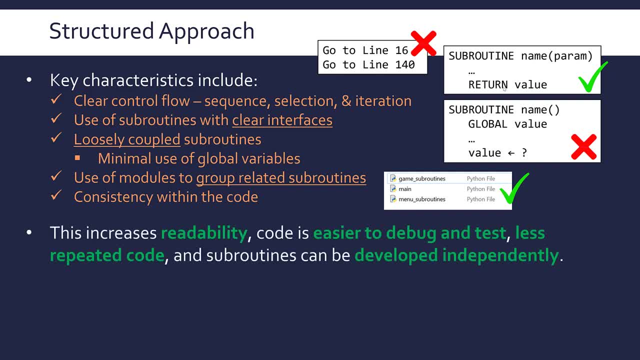 parenting makes it more readable, Which is really one of the purposes, one of the advantages of following the structured approach: that it makes it more readable, makes the code easier to understand. Now, also, if you've got these nice chunks of code in subroutines, if each subroutine is independent and 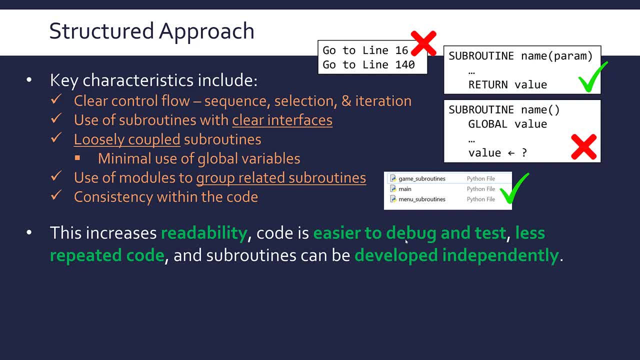 loosely coupled to debug it. you just focus on that one subroutine and you can test it using just that one subroutine. It can really break stuff down and focus on individual areas, not having to test the entire code because it you haven't structured it very well and 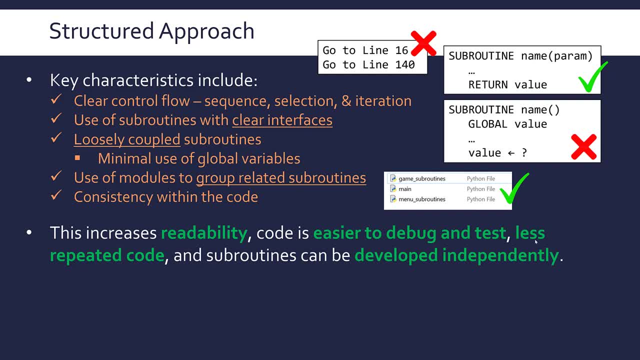 These are subroutines- generally leads to there being less repeated code. you just define it once and call it whenever you need it. you're not copying and pasting the same code again and again and Because the subroutines are ideally loosely coupled and pretty independent. 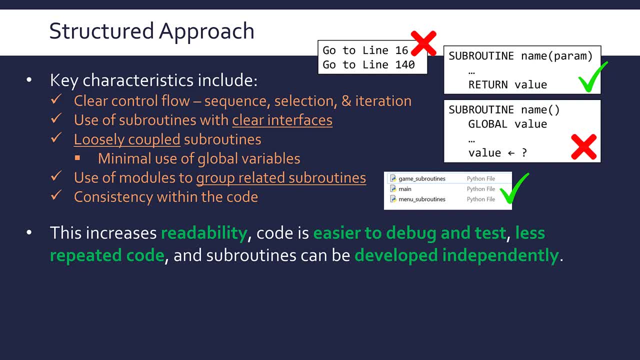 That means, if you've got more than one programmer working on this project, They can take their own subroutines, work on them on their own and then at the end Combine them and it should all fit together. Ideally, nice and well. Now, despite this being a very popular approach to programming and it's what you get taught, 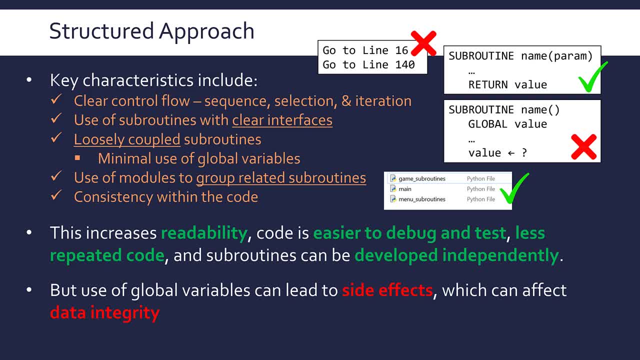 Where everyone gets taught. essentially, Criticisms of this approach are that because global variables are not banned, necessarily you can use them. They can lead to side effects, where one Subroutine affects another subroutine Unintentionally, and these bugs can be really really hard to fix because you're not always sure. 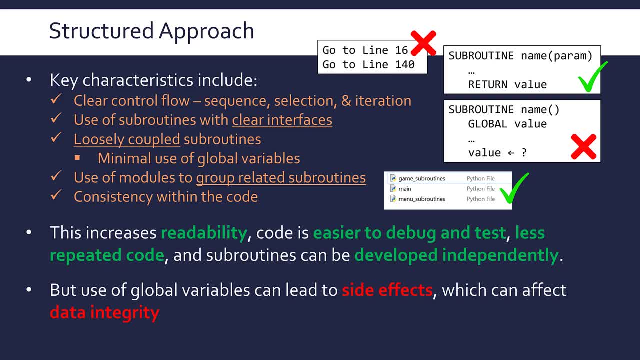 Exactly what's causing it, Especially if you've got Maybe hundreds of subroutines working together and this issue can affect data integrity. There aren't- there isn't- much protection of data within this system, which, when you compare it to object-oriented, Where you can encapsulate data and keep attributes private, is quite a stark contrast.